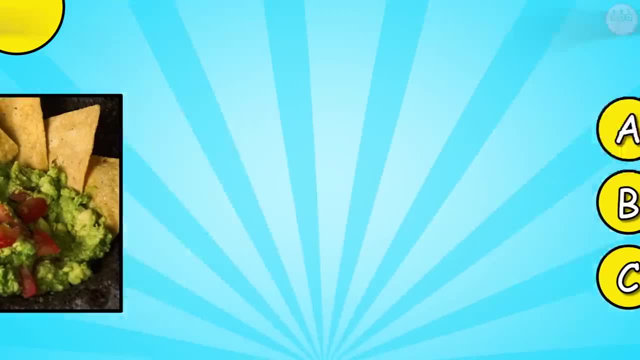 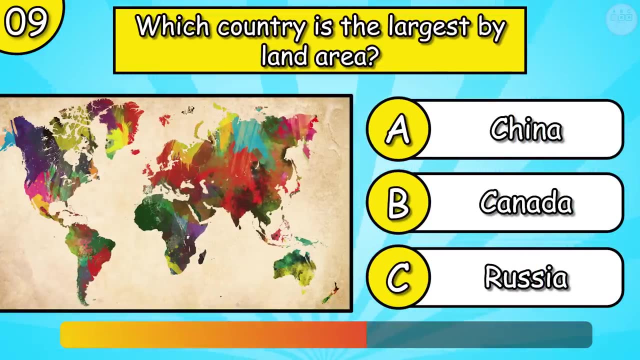 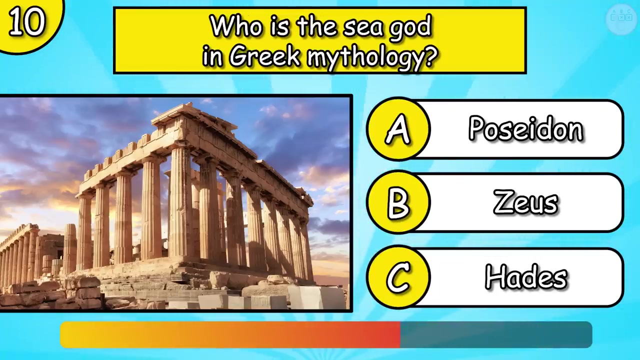 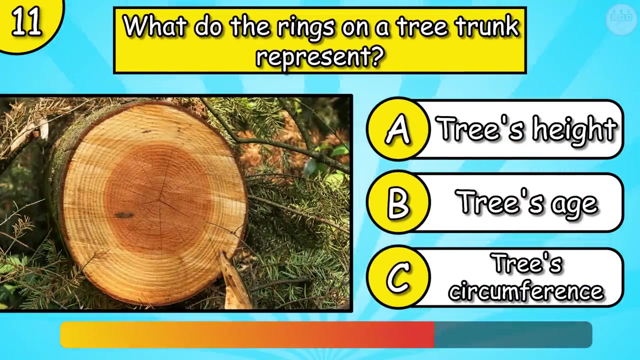 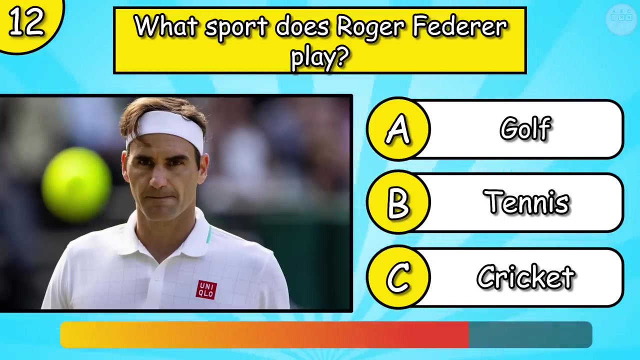 Venus, Avocado. Which country is the largest by lamp area? It's Russia. Who is the sea god in Greek mythology, Poseidon. What do the rings on the tree trunk represent? Tree's age. What sport does Roger Federer play- Tennis? Which of the following is a brass musical instrument? 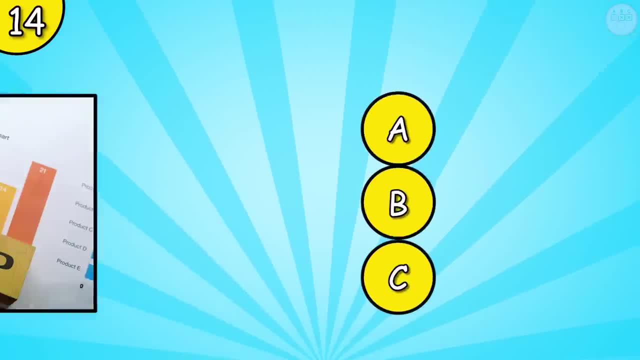 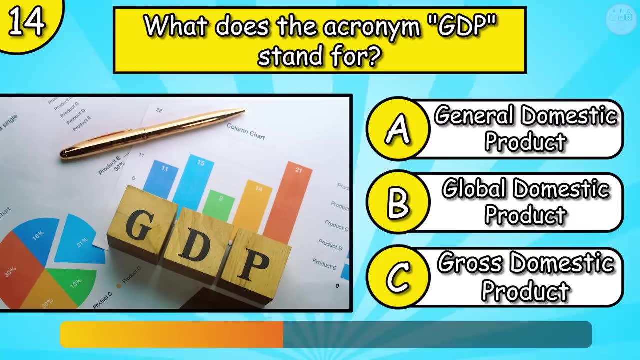 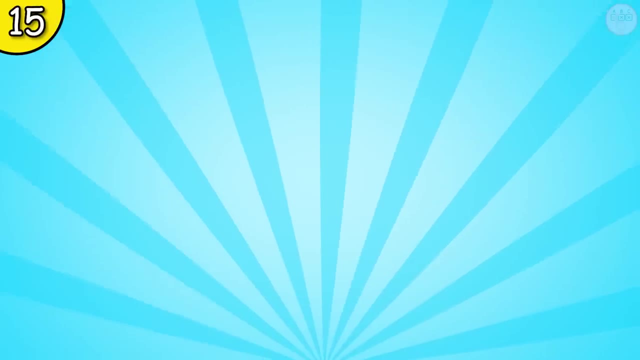 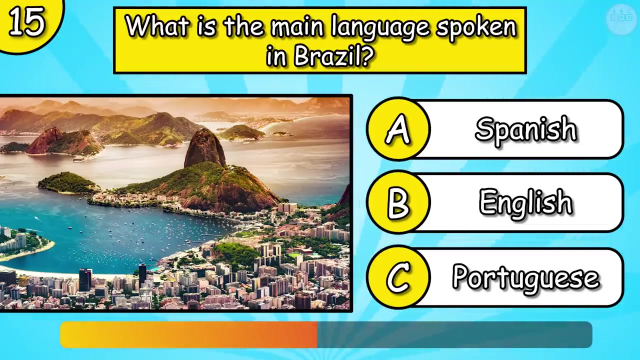 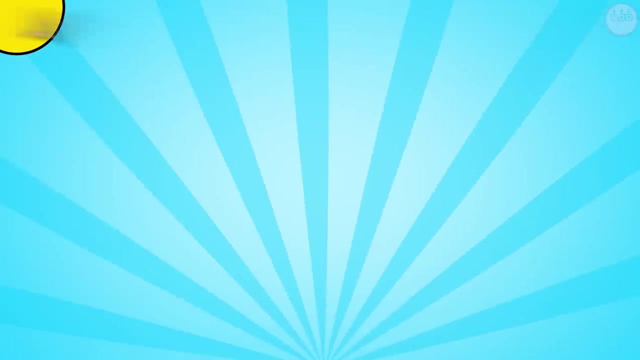 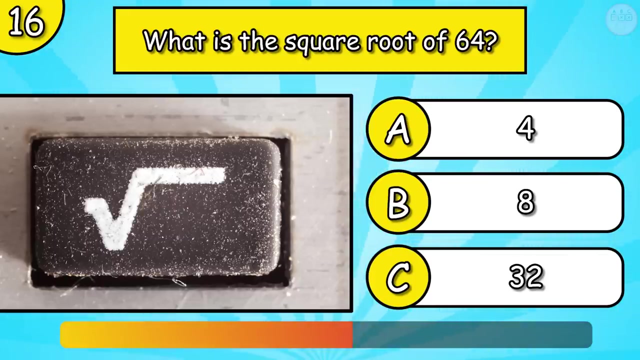 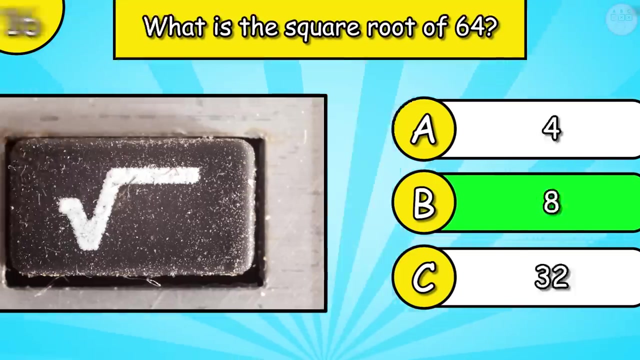 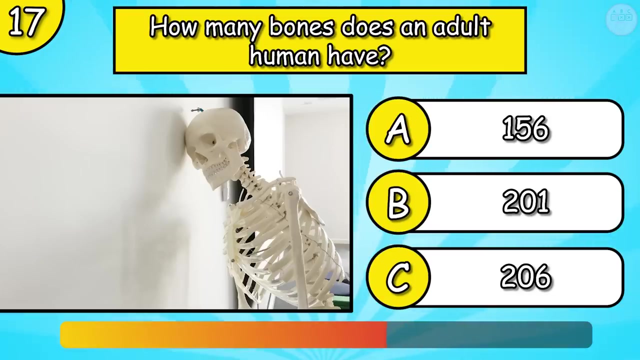 Trombone. What does the acronym GDP stand for? It's Gross Domestic Products? What is the main language spoken in Brazil? Portuguese. What is the square root of 64? Eight? How many bones does an adult human have? 206. What is the largest continent by land area? 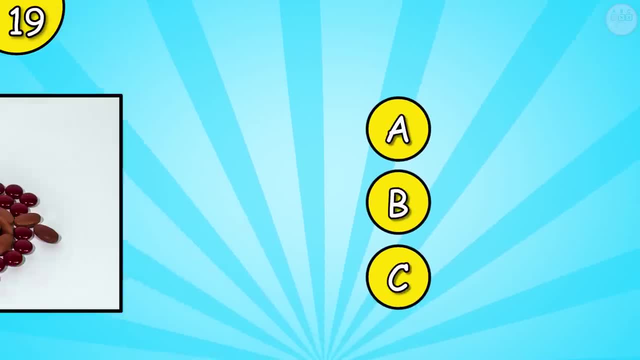 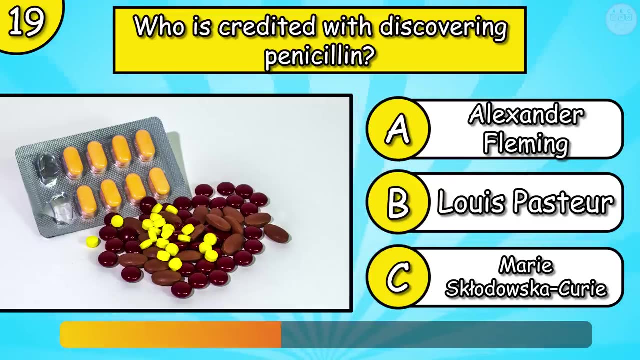 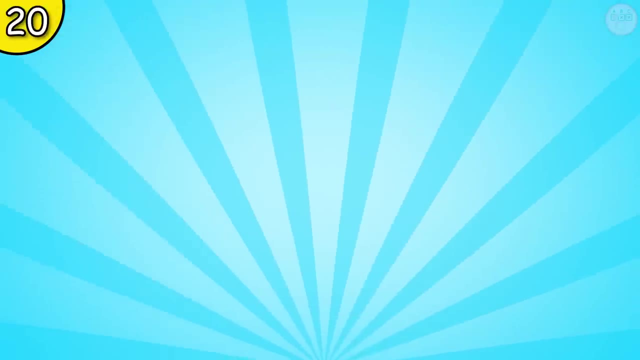 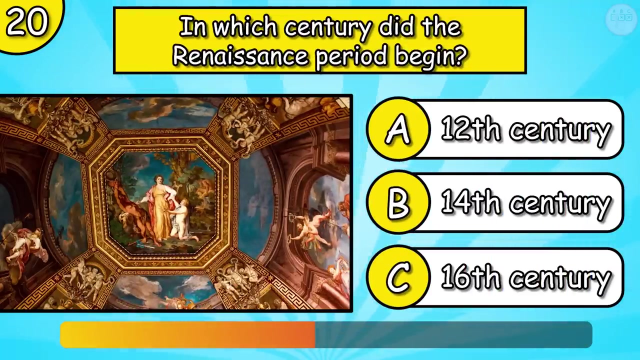 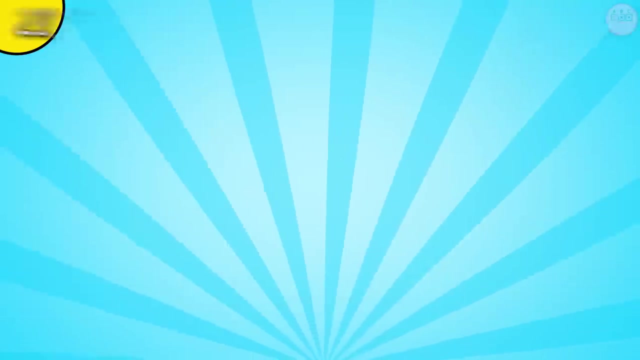 Asia. Who is credited with discovering penicillin? Alexander Fleming. In which century did the Renaissance period begin? In 14th century. In which century did the Renaissance period begin? In 14th century? What is the largest island in the world? Chapter 2: 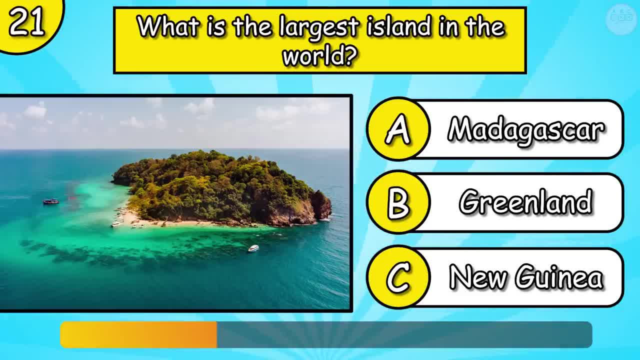 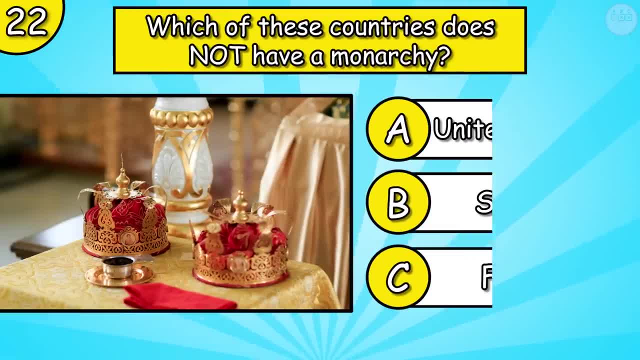 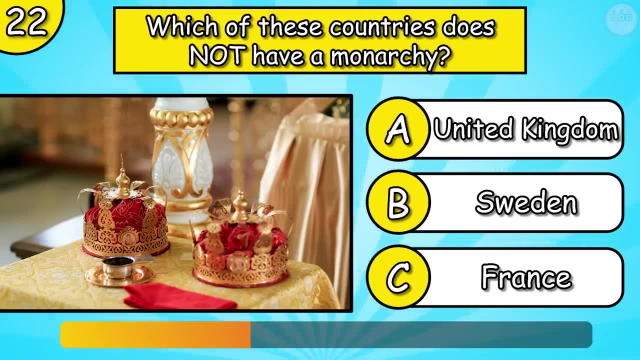 What is the corporation of the Constitution of France, Chapter 3? Which country has the most others in the world? It's Greenland. Which of these countries does not have a monarchy? Do Gen guy like to think of the capitals as ruling? France Estate. 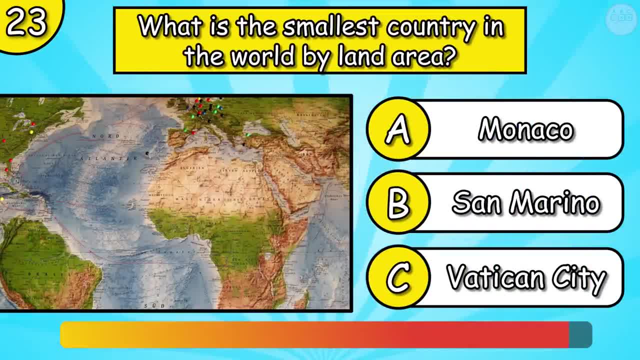 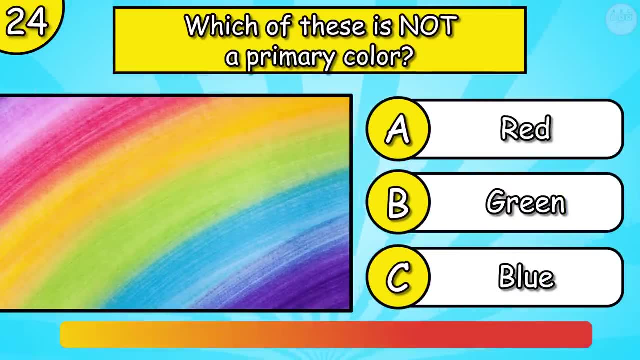 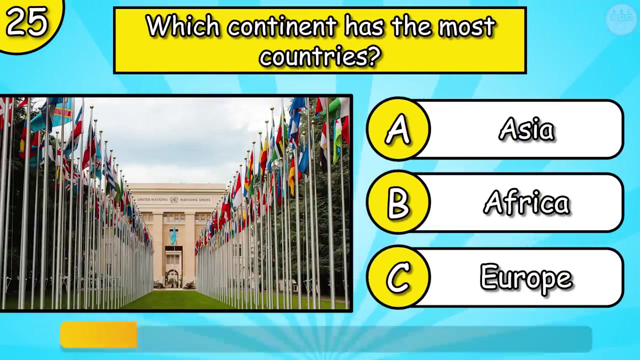 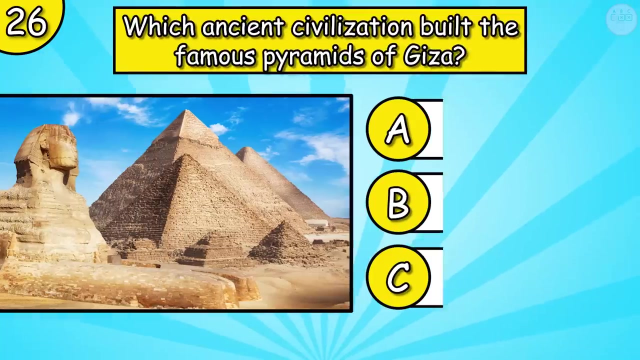 Is there aresident that offices properties in France, Ben Autry. what is the smallest country in the world by land area? it's Vatican City. which of these, is not the primary color green? which continent has the most countries? it's Africa. which ancient civilization built the famous pyramids of Giza? 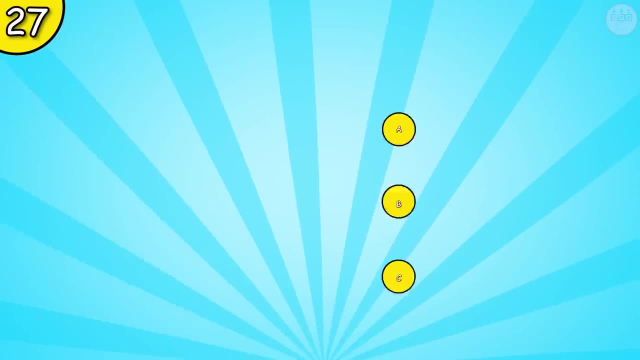 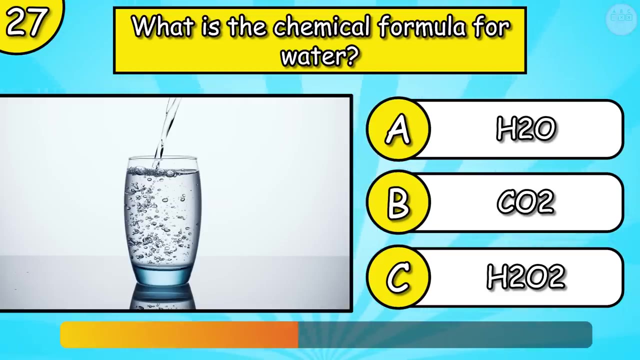 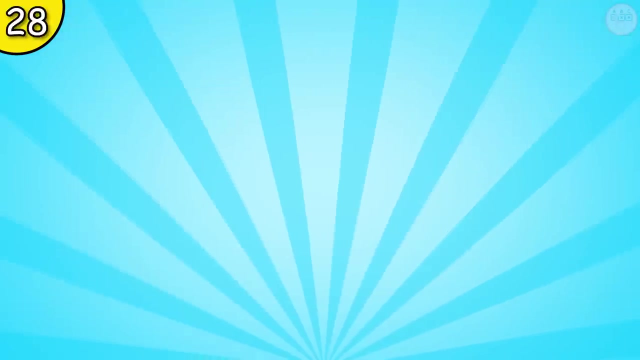 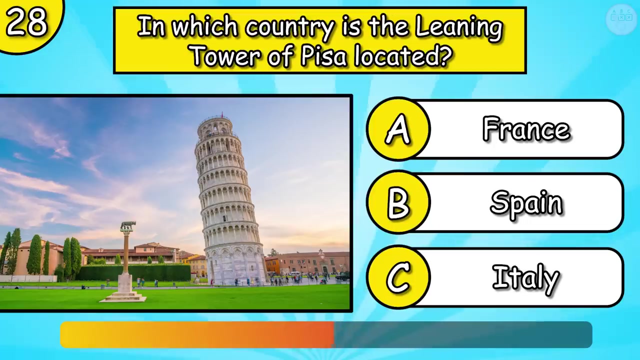 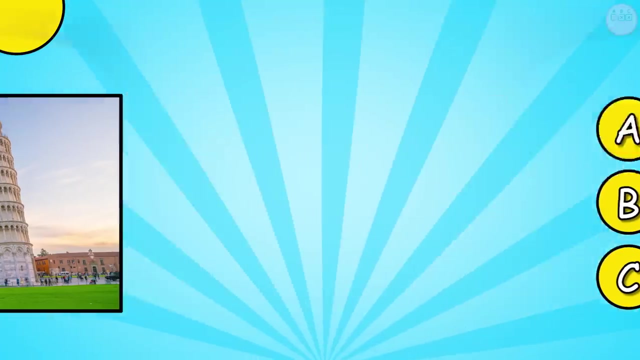 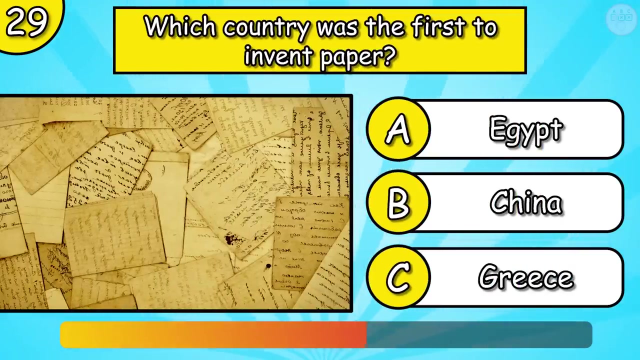 Egyptians? what is the chemical formula for water, H2O? in which country is the Leaning Tower of Pisa located in Italy? which country was the first to invent paper? China. what is the hardest natural science? what is the hardest natural science? what is the hardest natural science? 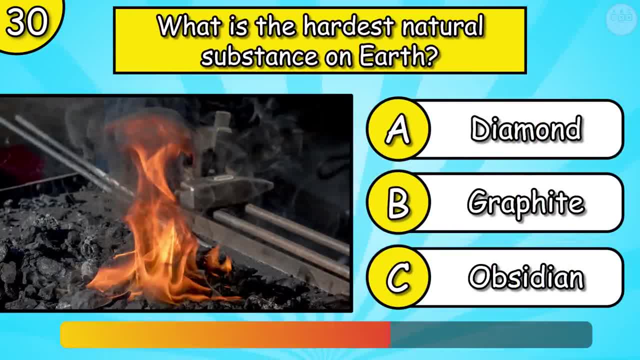 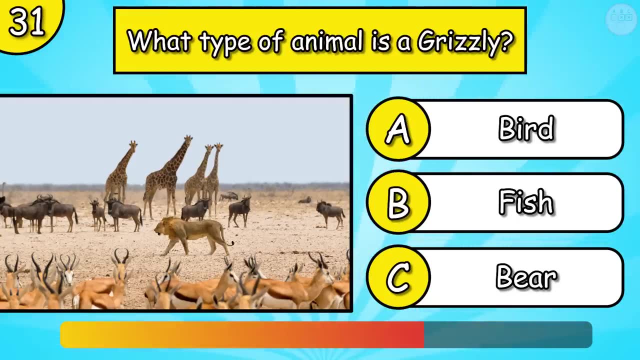 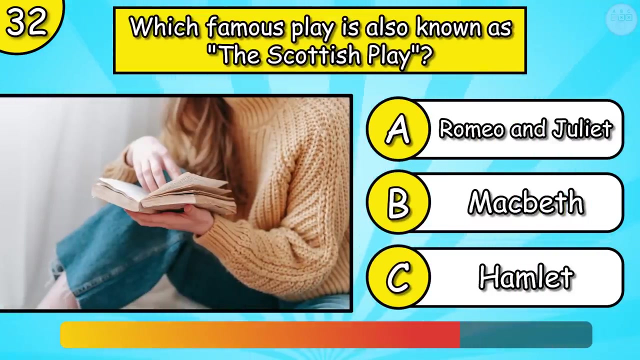 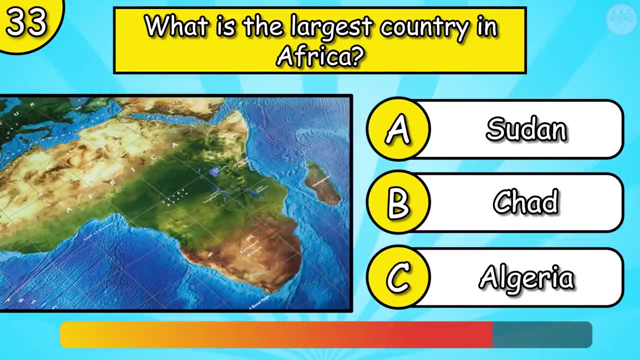 what is theаша? what is the hardest natural substance on Earth? it's diamond. what type of animal is a grizzly Bar? which famous play is also known as the Scottish play? it's Macbeth. what is the largest country in Africa- Algeria. what is the largest gland in the human body? 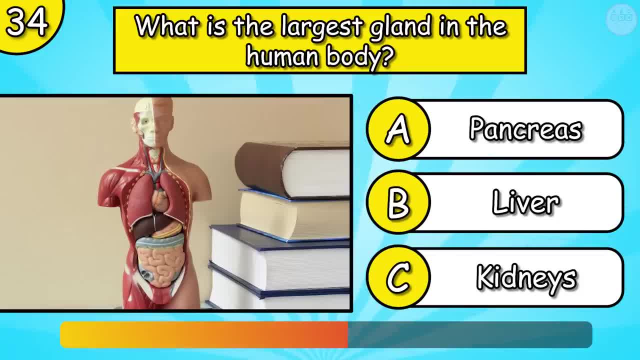 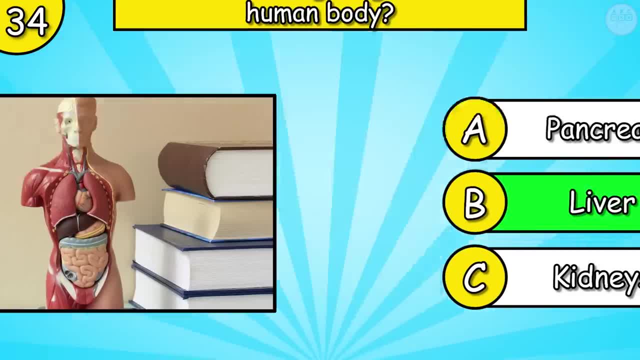 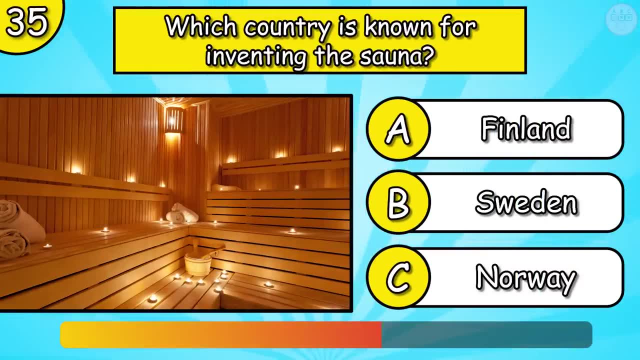 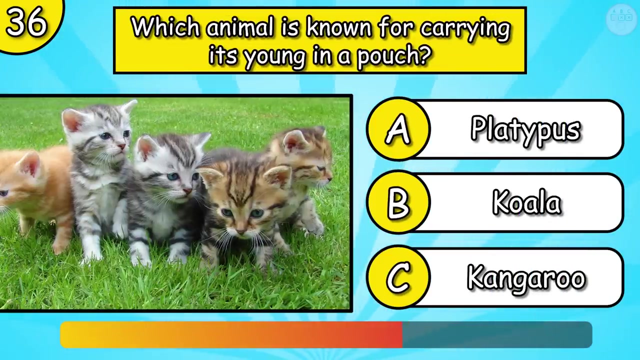 liver. which country is known for its inventing the sauna? Finland. which animal is known for carrying its young in the pouch? it's kangaroo. what is the official currency of India? India. what is the official currency of India? India. what is the official currency of India? India. what is the official currency of India? 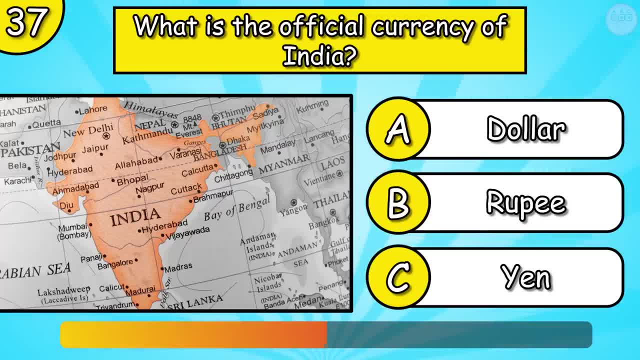 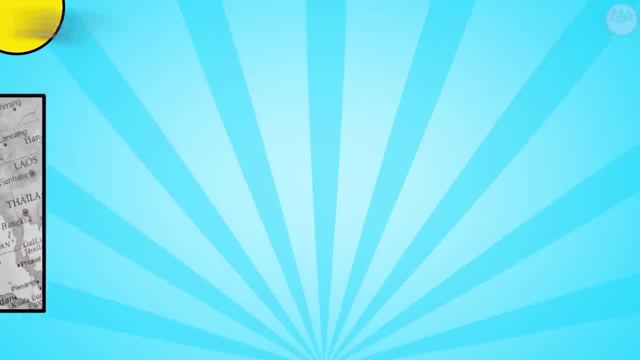 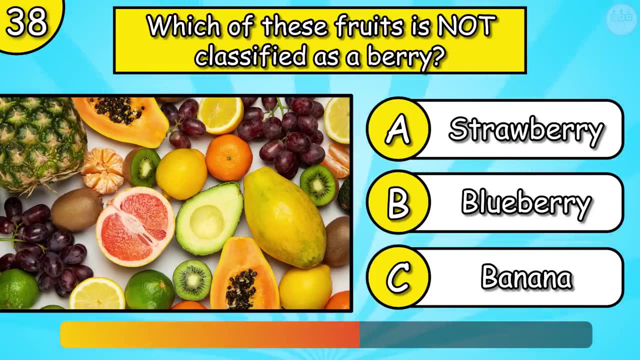 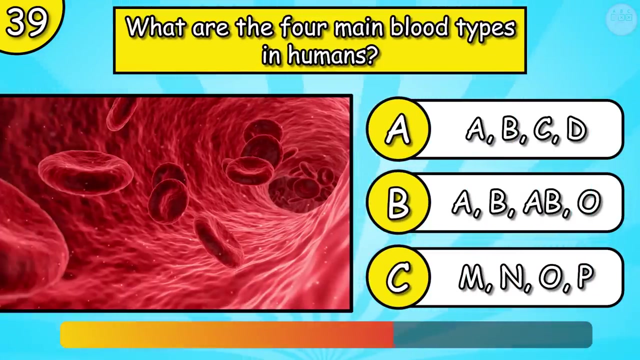 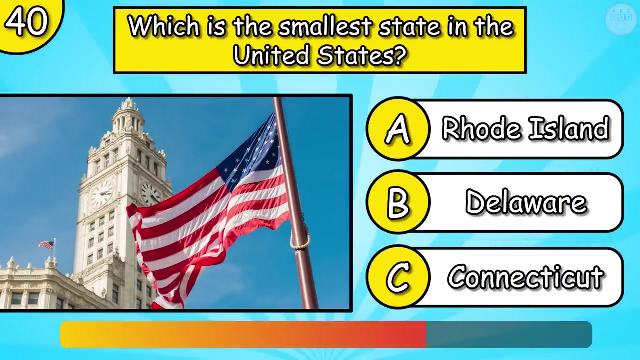 Which of these fruits is not classified as a berry? It's strawberry. What are the four main blood types in humans? A, B, A, B, 0. Which is the smallest state in the United States? It's Rhode Island. How many correct answers did you make. Let me know in the comments.